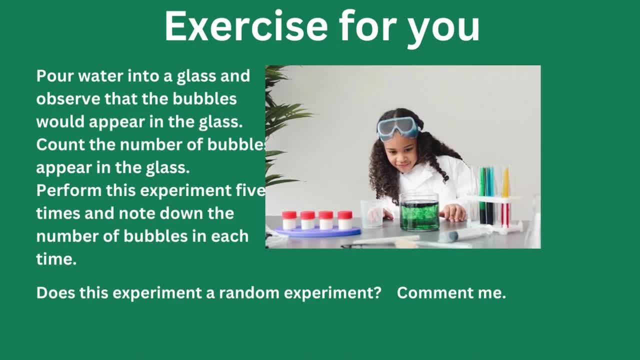 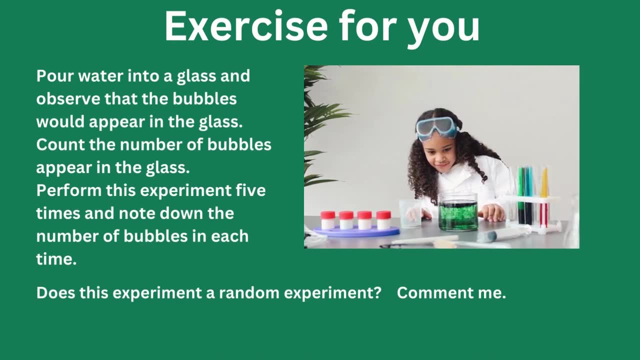 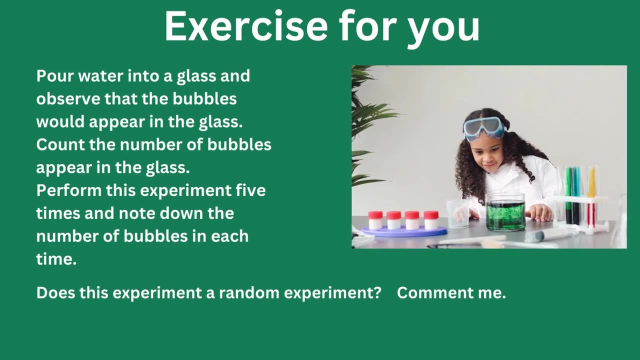 getting fixed result here. So this: now I am giving one exercise for you. You have to do this experiment to understand the random experiment. So let us start. Let us start: Pour water into a glass and observe that bubbles would appear in the glass and count. 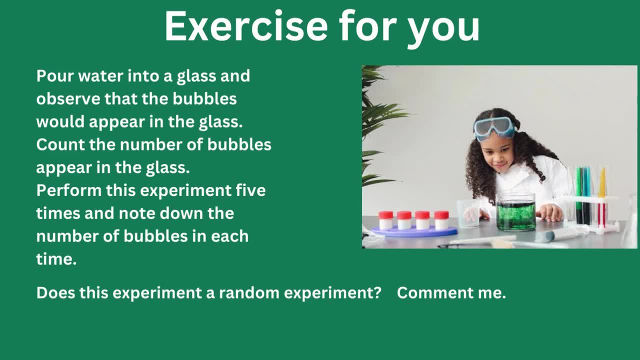 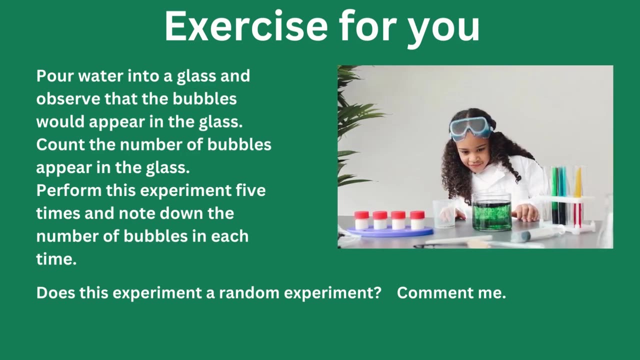 the number of bubbles appear in the glass. Perform this experiment five times and note down the number of bubbles in each time. So explore what you are getting from this experiment And also conclude that the experiment is a random experiment also. So let us start. 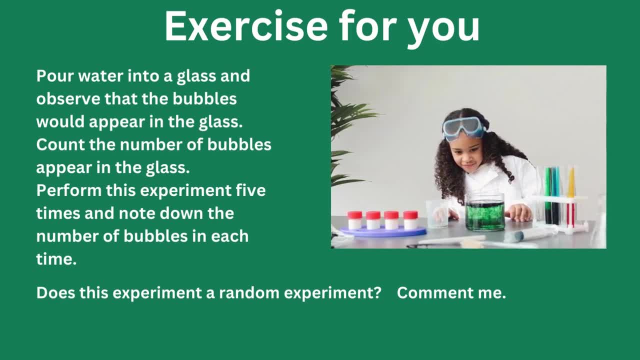 Pour water into a glass and observe that bubbles would appear in the glass and count the number of bubbles in each time. So observe that bubbles would appear in the glass and count the number of bubbles in each time. So let us start: Pour water into a glass and observe that bubbles would appear in the glass and count the number. 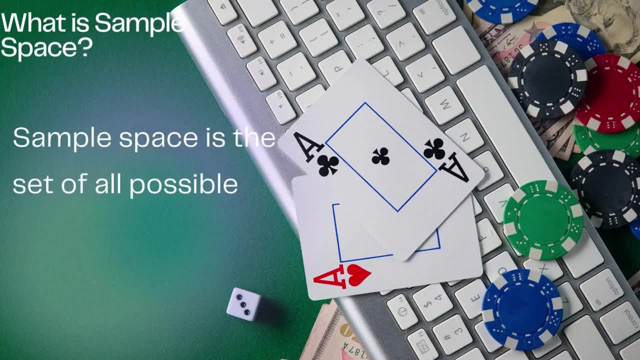 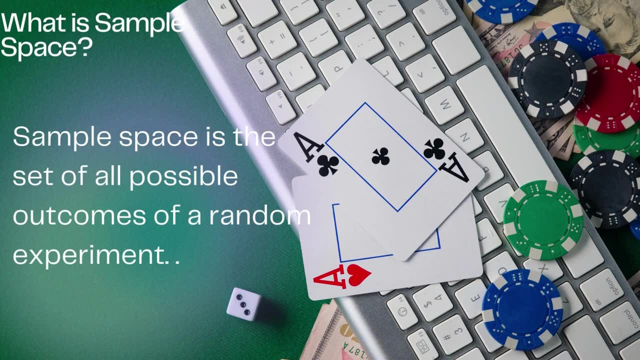 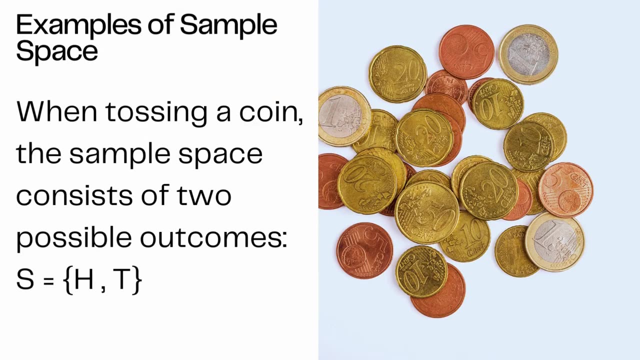 of bubbles in which to Berber can be changed from Здt cos and來到 the glasspan. If water is fried and experiments are left and stills, then you can observe the state of Sec空, whether the onunity ofح contact you or not. 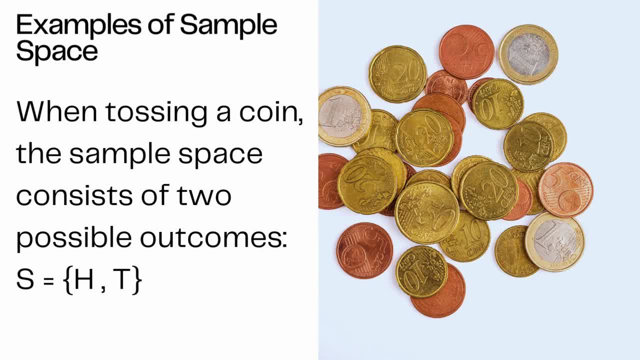 So now let us take a example. What is sample space? Sample space – Very few are possible outcomes for random experiments tossing a coin. so here we are tossing a coin, so we will get head either or tail. so that's why here we have listed all possible outcomes as a set S, so sample space is denoted by S. 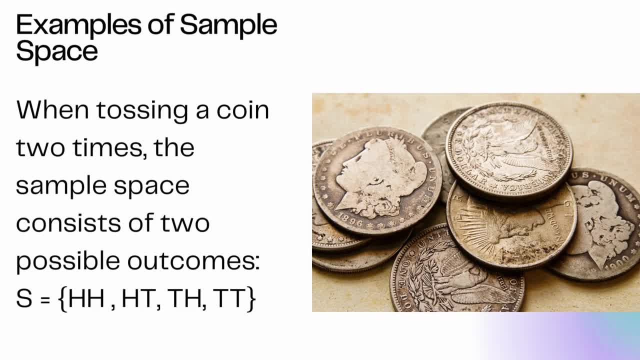 then. second example we will see when tossing a coin two times. so here we are, tossing a coin two times, so first time we may get head, then second time we may get head, or in the second possibility we will get first time head, second time tail or first time tail. second, 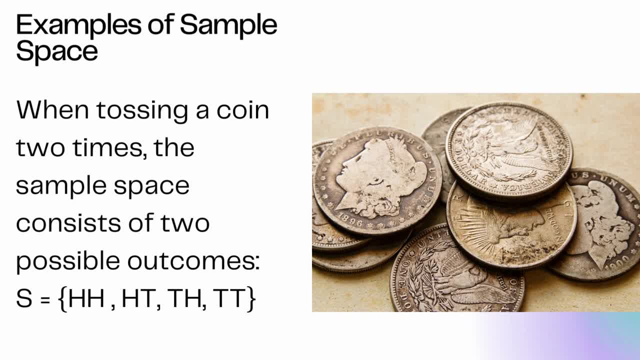 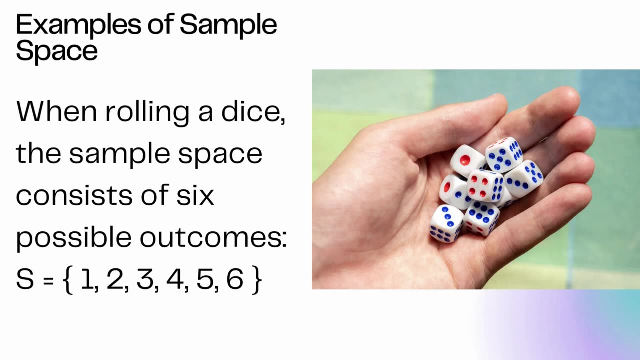 time head. and the last possibility is both you will get tails. so all these possibilities listed in the state of this as a sample space. then, third example of rolling a die. so when we are rolling a die we will get the six possible outcomes. so these are the numbers of dots on dies. so 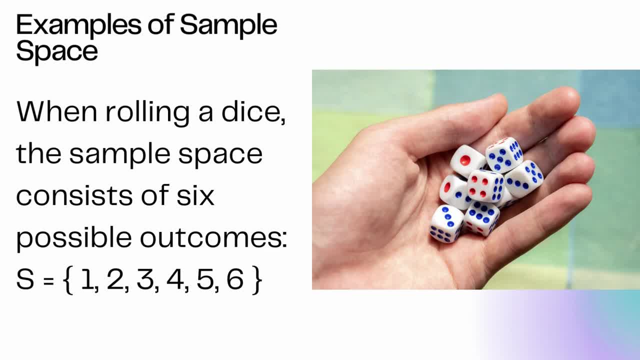 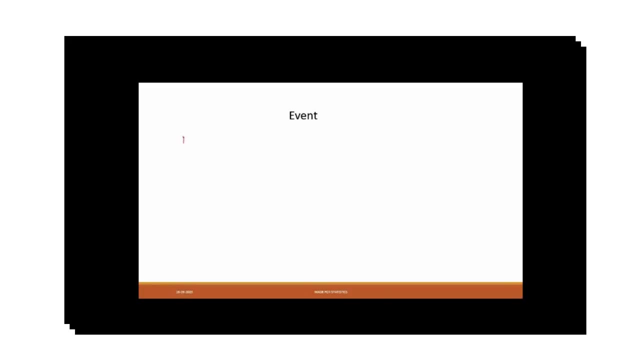 So this is denoted by S and which is equal to 1,, 2,, 3,, 4,, 5, 6.. So event is nothing but a subset of sample space. So I will write in definition: event is a subset of sample space. 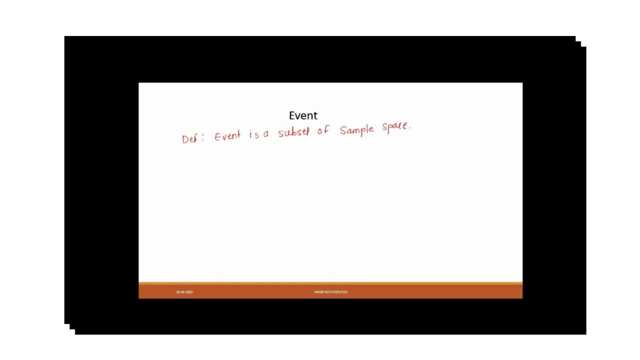 So in earlier example. so this three experiment we will take: First experiment is tossing a coin, Second experiment is tossing a coin two times And third experiment, rolling a die. So here I will define my event, A. So event can be defined by A. 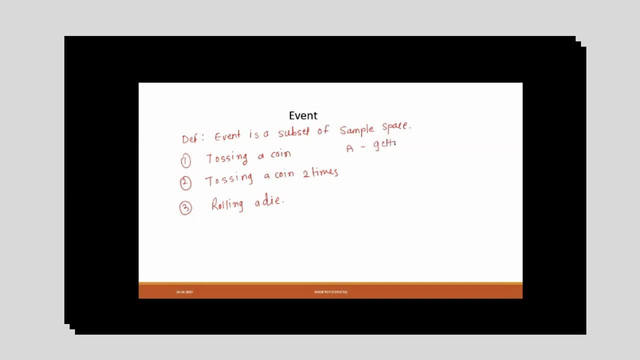 It's getting a head Then. so sample space, my sample space is so for this my sample space is head and tail. So for A I can write only head Right For then. second example: suppose my A I have defined, getting exactly two head. 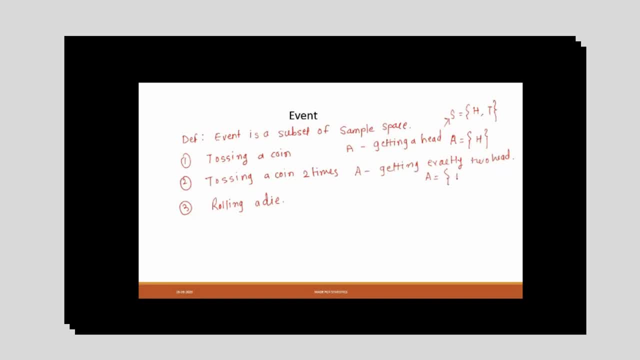 Then my A will be only one element, because I want exactly two head Then rolling a die. I will define my event So it's mostly So. for the second question: it is defined and you have to check what element are coming. 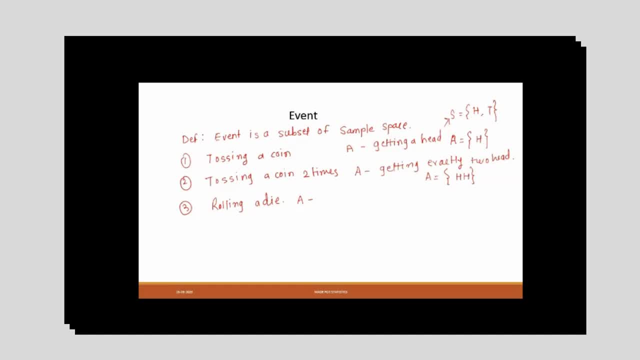 If this, a or its, defined in the equation like what is event, And you have to give, prepare this set of event, What element will be there And you can calculate the probability on the basis of that. Okay, so here I will define in third example: event. 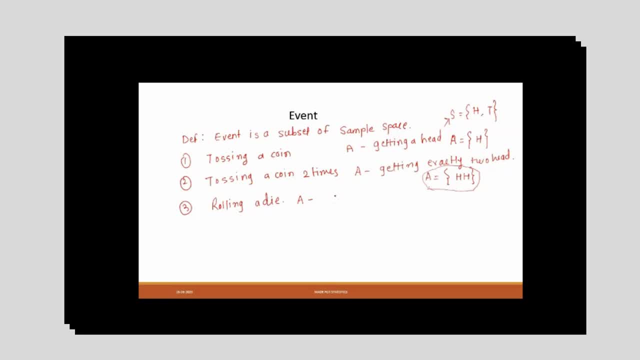 A is equal to Okay, So I want to consider only A in the third example. So it will be there. the number of dots appears on die are multiple of 7. so now tell me, if my sample space is 1, 2, 3, 4, 5 and 6, then for a there is nothing, so i can define a as a empty set also. 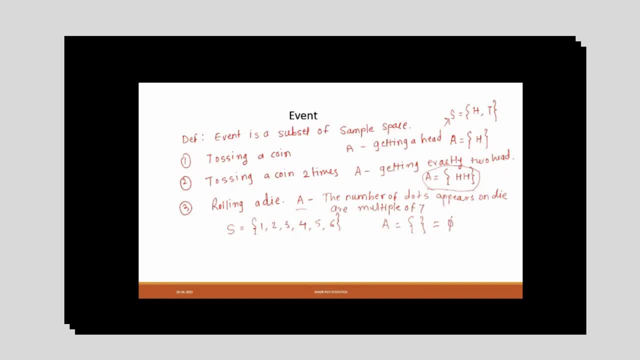 it can be written by 5, right? so this is my empty set, this set also known as impossible set. also, suppose i will define my event b as a. the number appears on die is less than 7.. so why 2, 3, 4, 5, 6? all are less than 7. so my b is nothing but 1, 2, 3, 4, 5 and 6. so this is nothing but my. 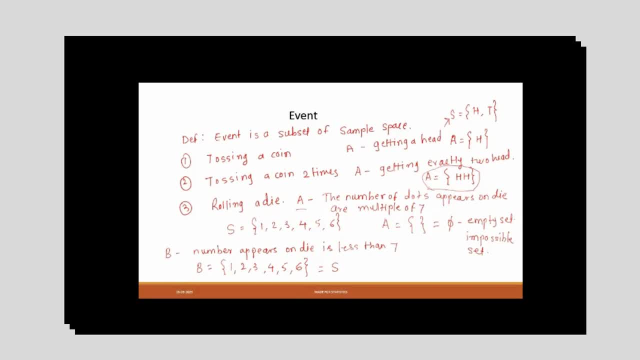 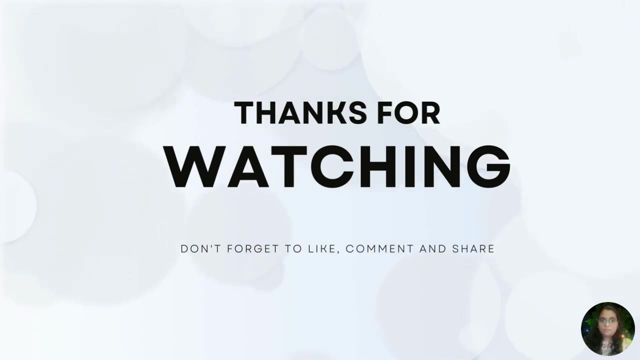 s. so whenever event is equal to sample space, then you can say: this is your sure set. thank you for watching. don't forget to like, comment and share. please subscribe and click on bell icon so that you will get all notification of my videos. also in the next video i am going to. 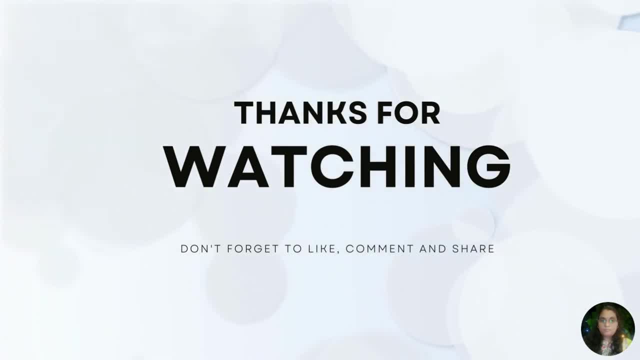 discuss classical approach of probability, axiomatic approach of probability and few example on computational of probability. so thank you, bye, bye, see you.